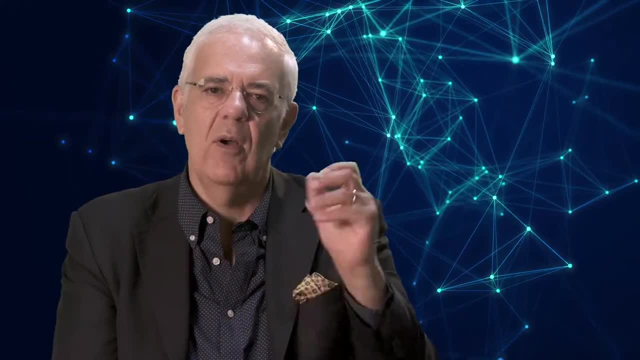 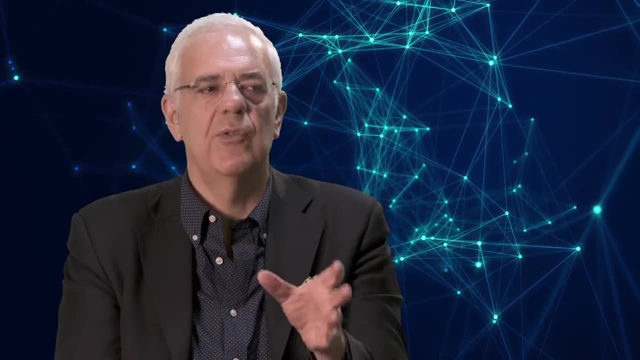 we mean the assignment of a time law along the geometric path. Now we'll be solving two kinds of problems: the point-to-point motion and the motion through the sequence of points, And in doing this we also want to be able to account for the dynamic constraints. 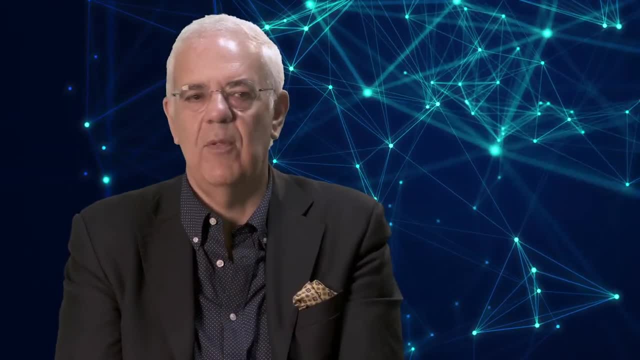 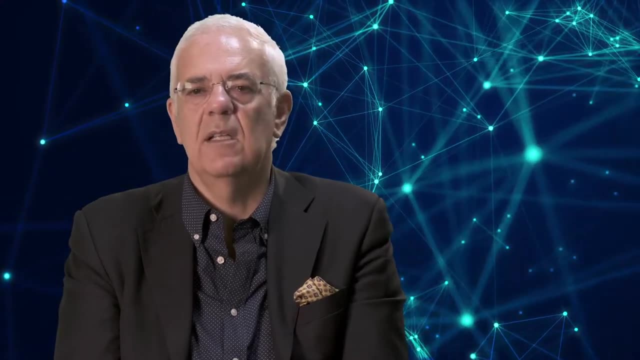 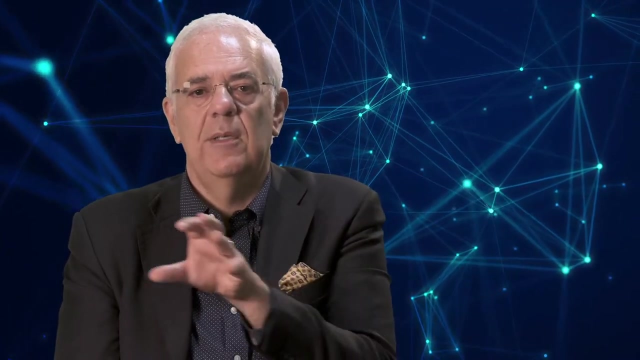 given by the torques to be exerted along the motion by the robot manipulator. How do we want the trajectory planning algorithm to be? We want this trajectory planning algorithm to be simple in terms of a reduced number of parameters. So, for instance, the initial point and the final. 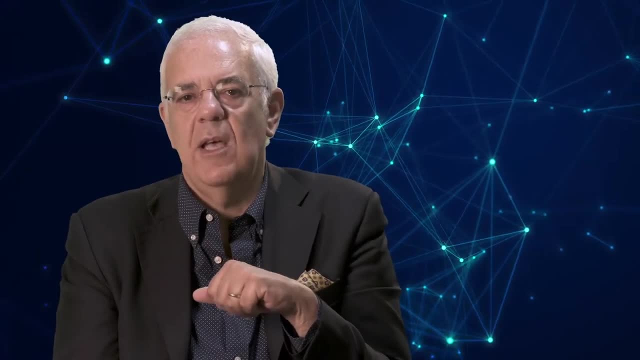 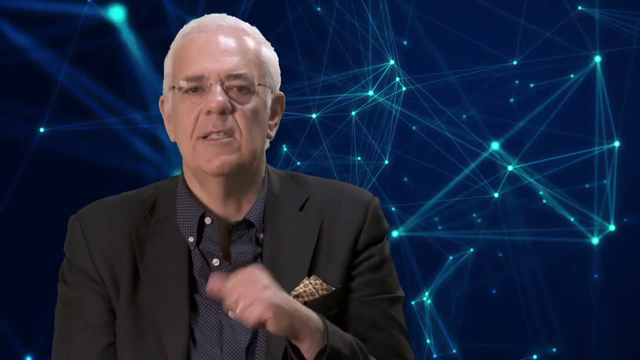 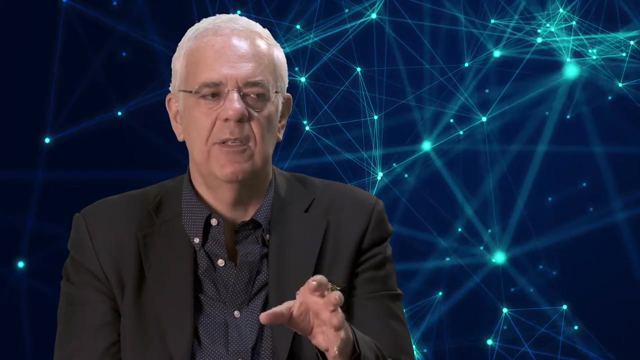 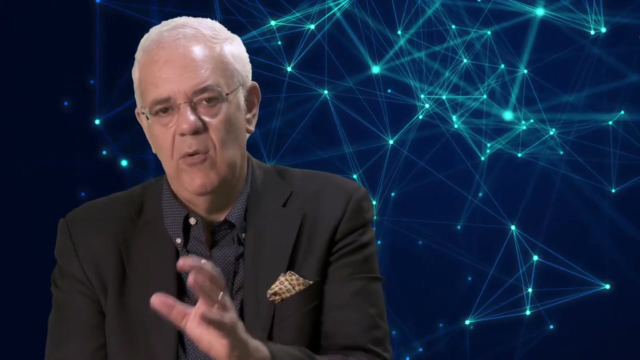 point of the trajectory planning algorithm should be equal to the number of parameters. We want an analytic expression and interpolating function for the time law We specify the final time, although in industrial setting this is not usually allowed for the user- and also we want to be guaranteeing the continuity of velocity and acceleration along, along, along the path. We can solve the problem in the joint space, as we'll be doing in this unit and in which typically we solve the inverse kinematics and then we generate the reference. 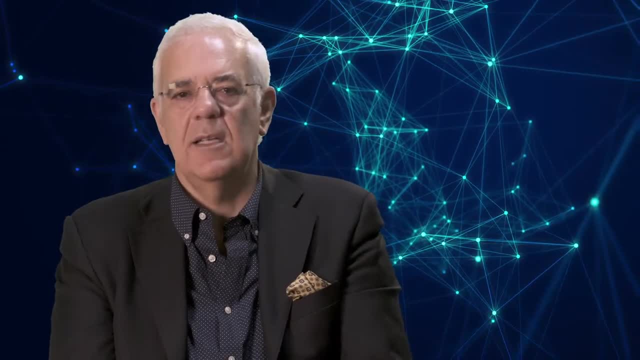 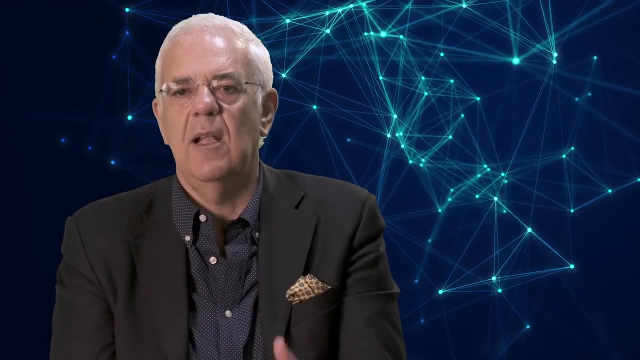 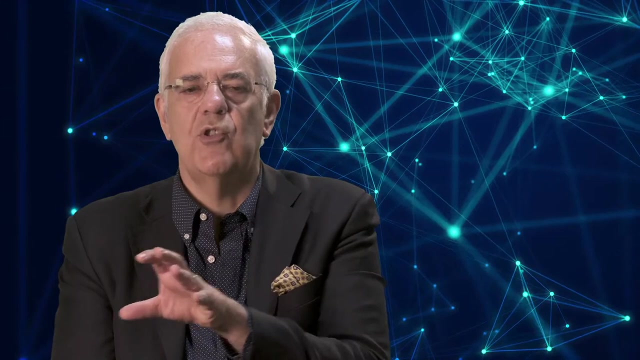 For the control schemes in joint space. otherwise, in the second unit, we'll be solving the problem in the operational space, in which we'll be accounting for the natural constraints like object singularities, redundancy and so forth. So let's start with the problem of the point-to-point motion, and I want to 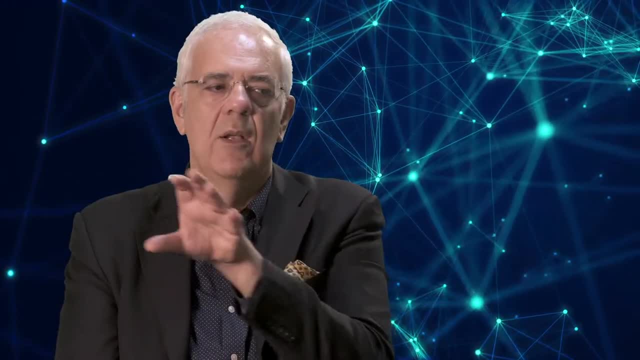 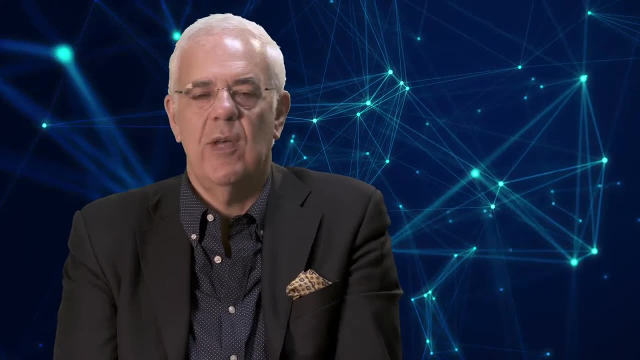 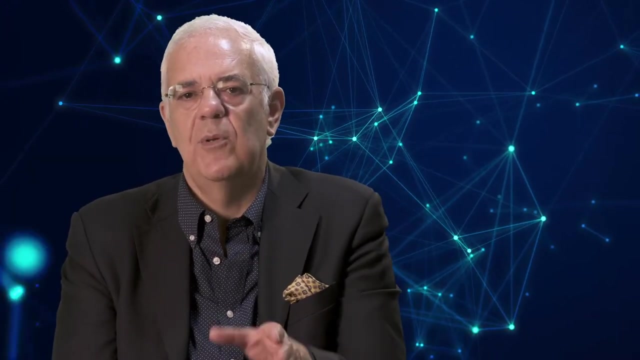 move the joint from initial position qi to a final position qf, and I want the generate trajectory to be smooth and also I want to guarantee the continuity of velocity accelerations. besides the position and more importantly, I want that the computational is simple, so the algorithm must be computationally cheap. Let's start with the 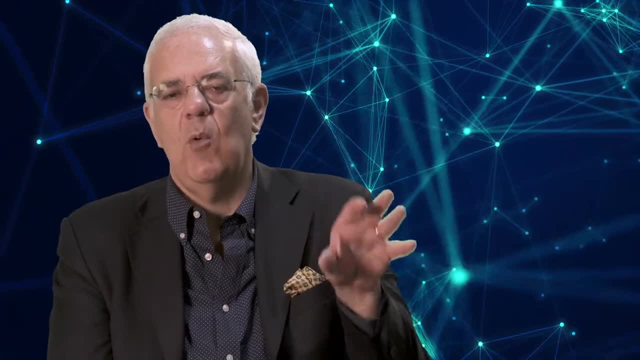 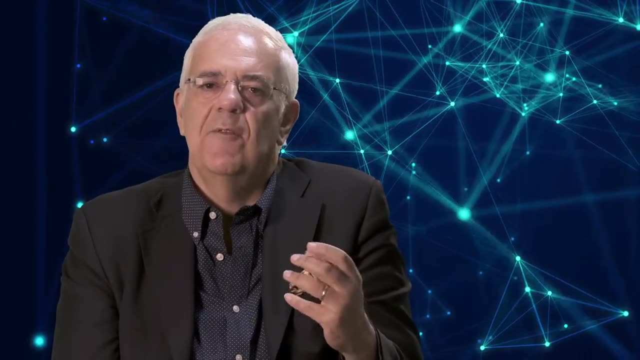 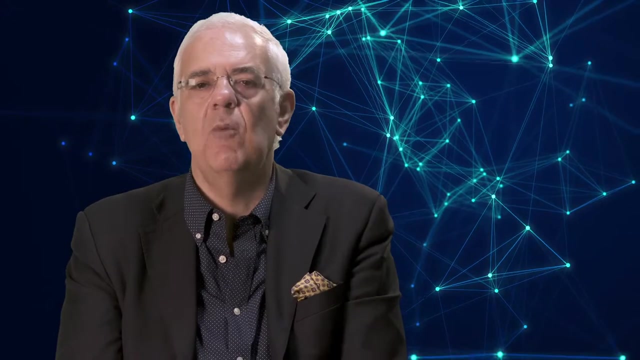 point-to-point motion. If we want to interpolate from qi to qf, we can use a linear blend, but then we won't be able to specify the velocities. So if we want to specify the initial and final velocity, the solution goes through adopting a cubic polynomials with: 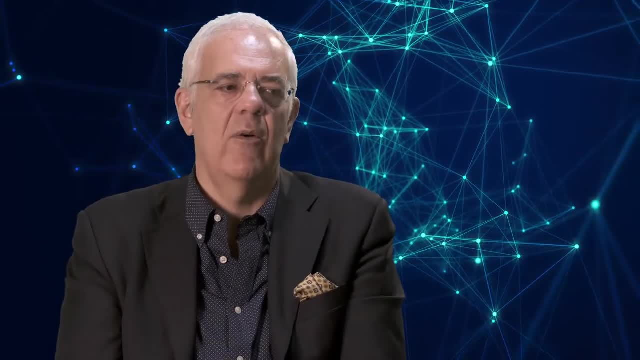 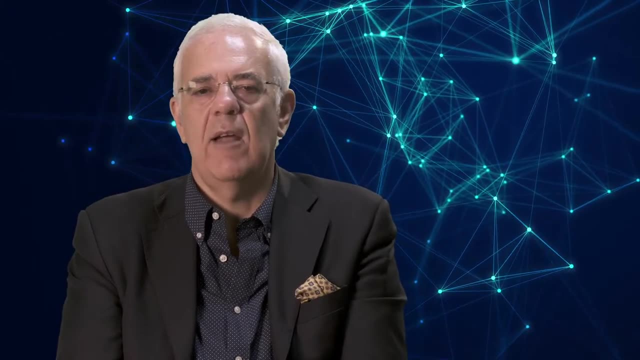 four coefficients. so we have a system of four equations in four unknowns, which can be simply solved for to compute the interpolating motion- What if we want to interpolate? and guaranteeing also a given value of initial acceleration and final acceleration. The order of the polynomial. 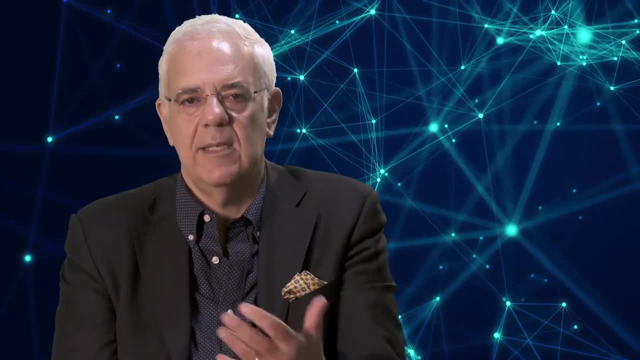 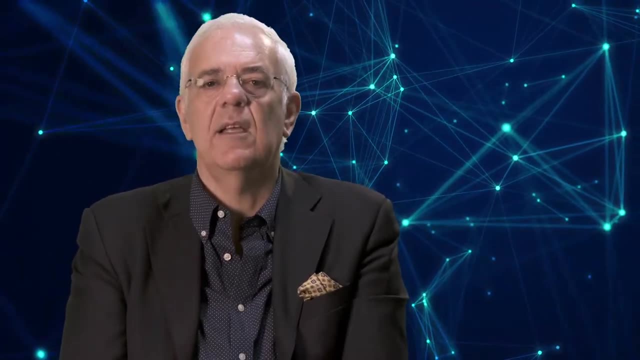 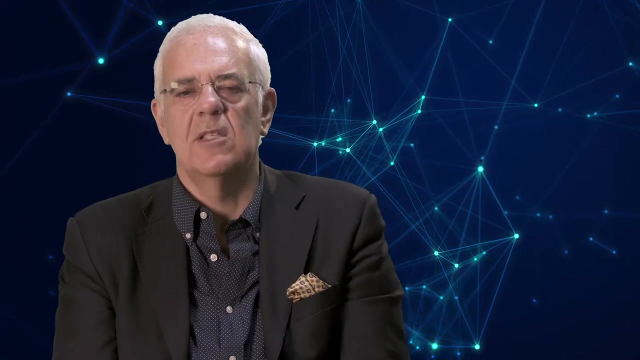 grows from three to five and with the quintic polynomial, six coefficients, six unknowns, six unknowns. so in six equations we can solve the problem. In the industrial setting there is a technique which is competitionally cheaper, And this consists in adopting the trapezoidal velocity profile. It's a very simple concept. 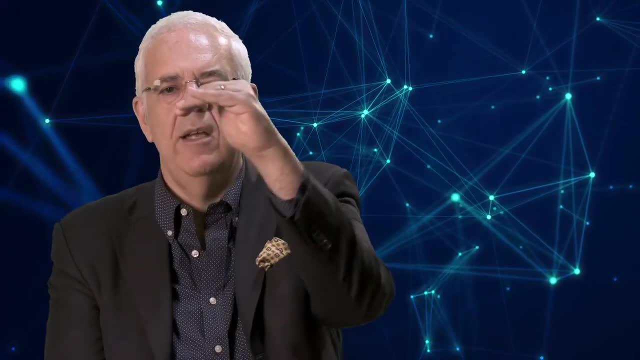 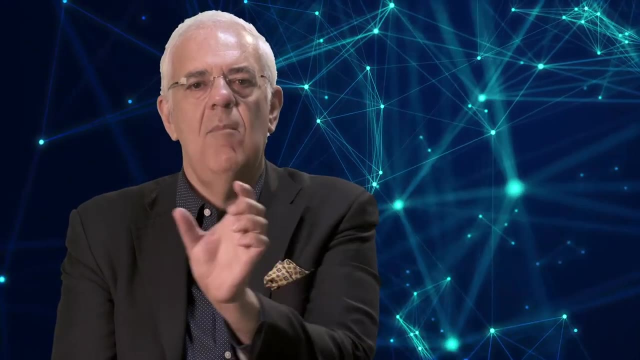 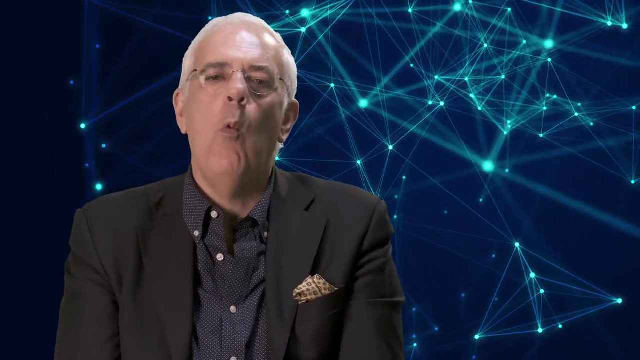 You accelerate to the top of your velocity, then you have a cruise and then you have a deceleration, and the actual mathematical way to solve the problem is to consider an acceleration time, a symmetric deceleration time, duration of tf minus tc. and then you have two techniques. One is to specify the 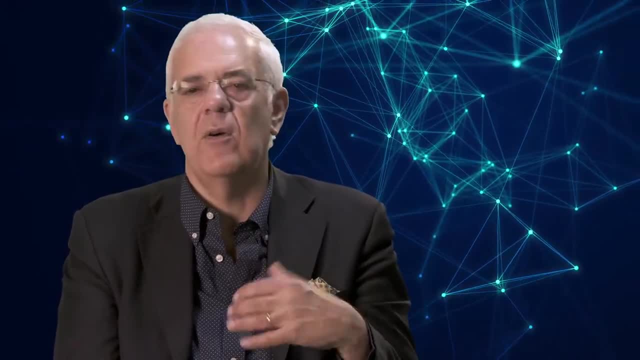 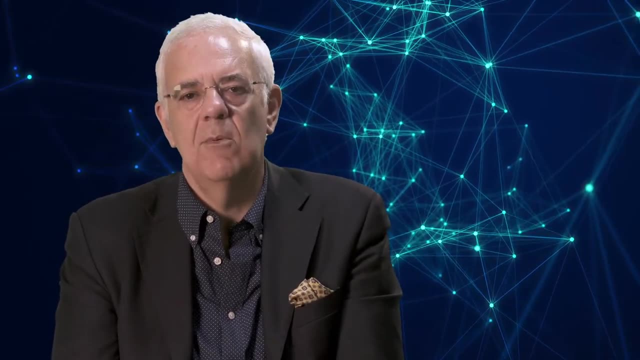 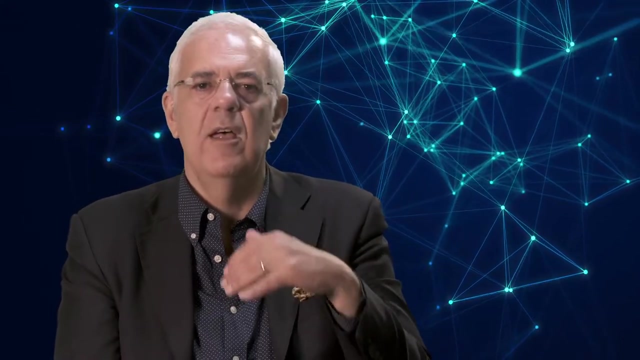 maximum value of acceleration, which, of course, must be greater or equal at four times the total stroke divided by the square of the of the final time, or specifying the maximum value of velocity, which, in this case, must be limited between the total strokes, time divided by tf and two times the total. 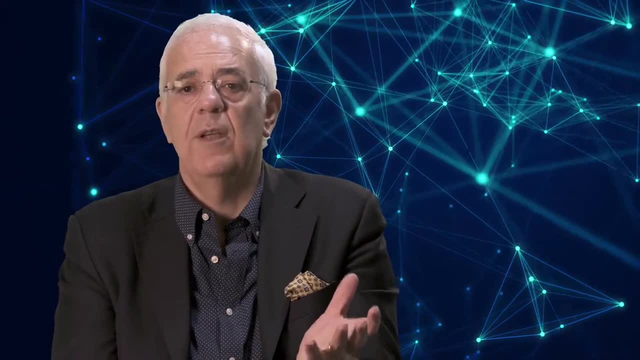 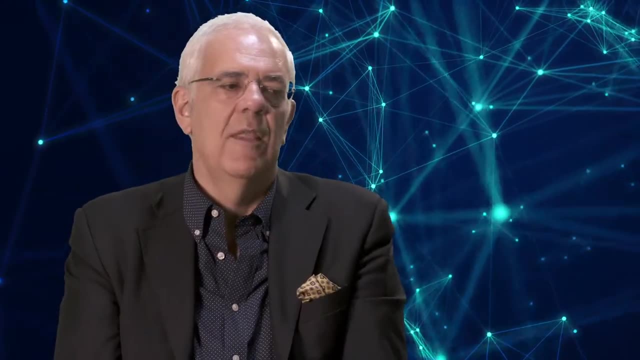 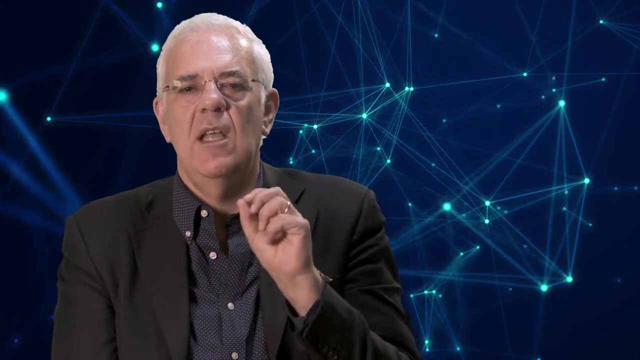 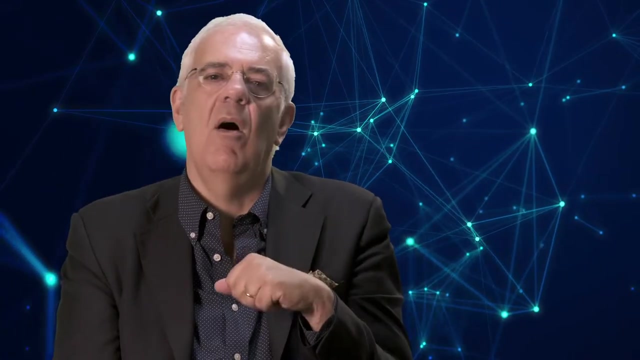 stroke divided by tf. This is fine for solving the point-to-point motion. Let's consider now the motion through a sequence of points. We'll be presenting four techniques. The first technique is basically to um, to interpolate through a sequence of points and in specifying the values of velocities. But you may wonder though, why not to consider a polynomial? 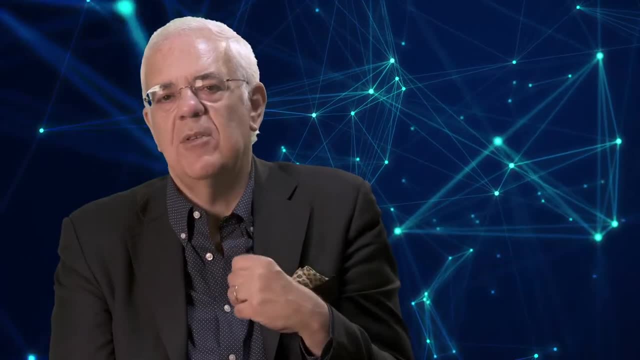 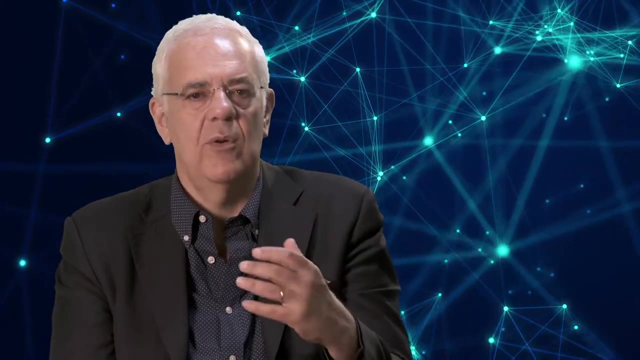 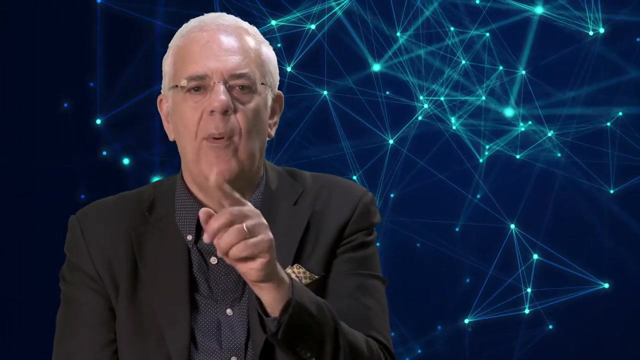 of order n minus one to solve this problem, because this will be will be coming computationally too heavy and also the degree, the degree of accuracy of the solution will will decrease as the as the order of polynomial increases. and if you want to change one point in the sequence, you have to 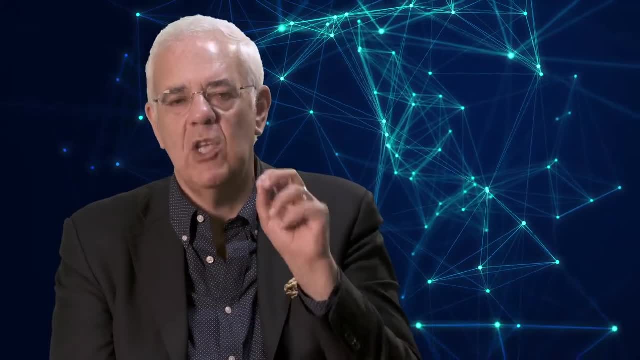 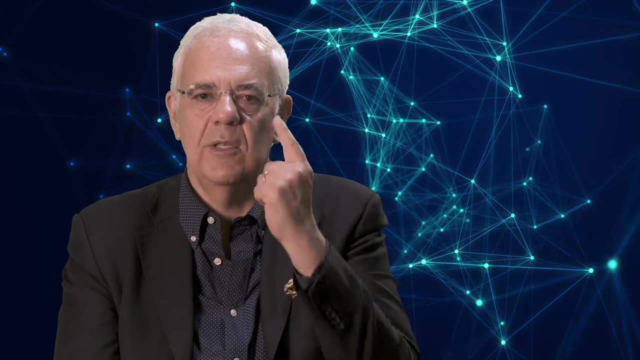 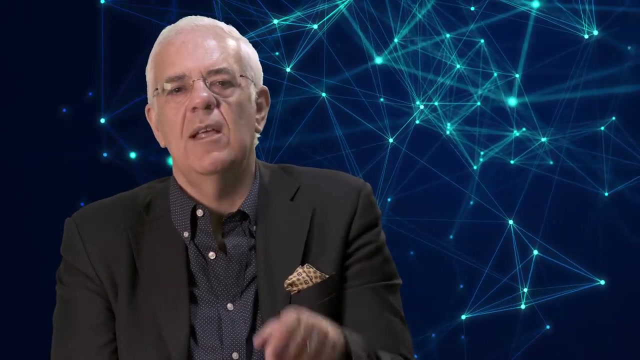 recompute everything. So let's consider n minus one cubic polynomial to interpolate, and just we specify the values of the velocities at the intermediate points, just guaranteeing continuity. So this is technique number one. Technique number two: we can compute those velocities as the simple average of the, as the simple, uh, the average sum of the. 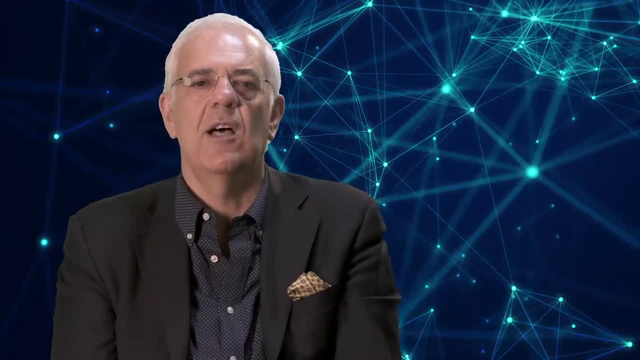 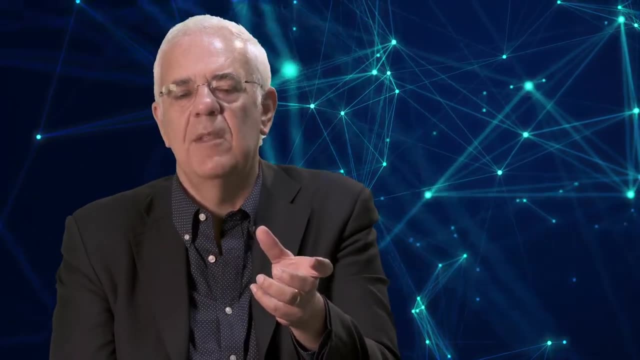 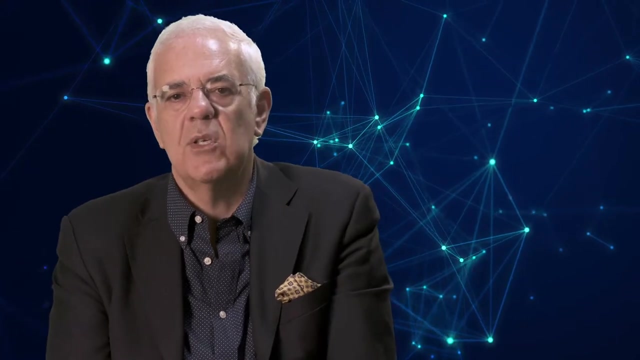 velocities in the previous time lapse and in the subsequent time lapse. We can do, we can compute this average, and if the two signs of the velocities are are disagreed, then we just set zero as a value. Now, this is to guarantee continuity of velocity. but you're also concerned with continuity of 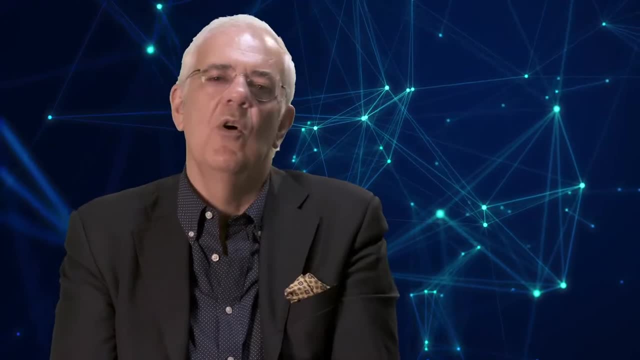 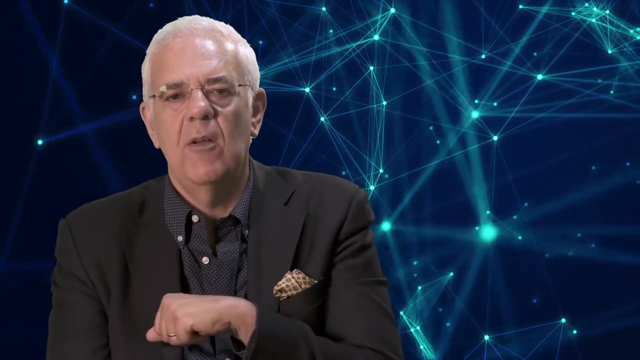 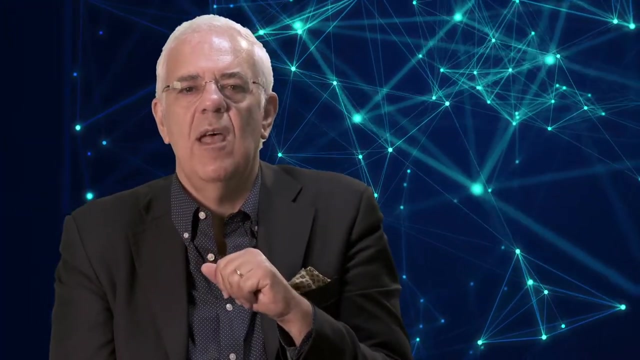 accelerations. and this brings us to the third solution, which is which is the so-called splines. What is a spline? Spline is uh, is a sequence of interpolating polynomial to the sequence of points, which which gave a smooth trajectory. Now, if you have n points, you can have four times uh, four. 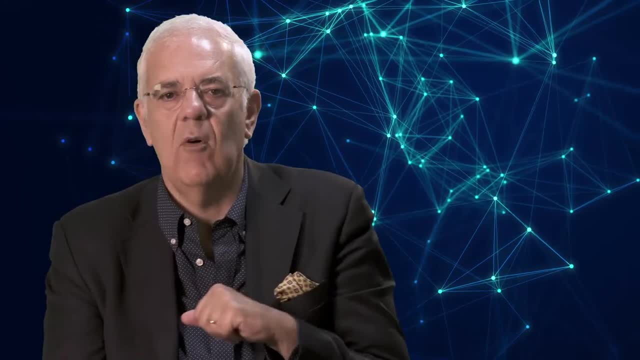 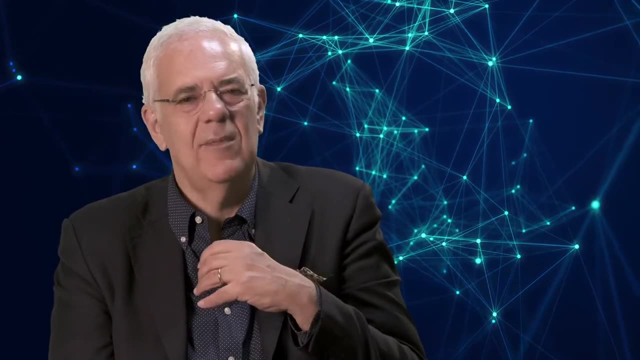 coefficients for each polynomial and n minus one polynomial, Then you have a square system of four n plus four equations in four n plus four unknowns. Then if you want to specify the initial and final acceleration, then you could use a fourth order polynomial, but this: 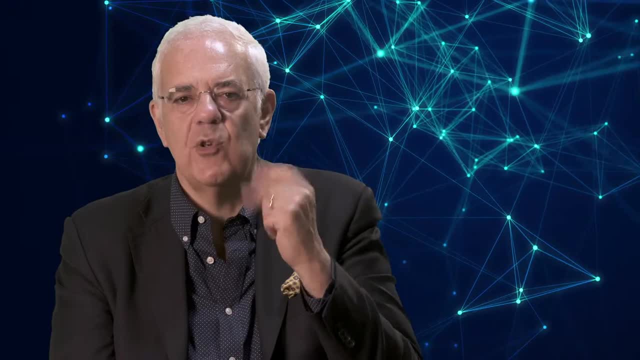 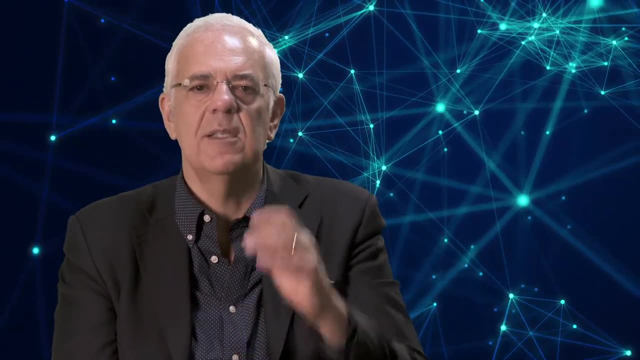 would would lead you to an asymptomatic solution. So, basically, other than considering this solution, we introduce two virtual points. We're not concerned with the actual position of those points, but we're just concerned with the time instant. and if we compute the whole system, we 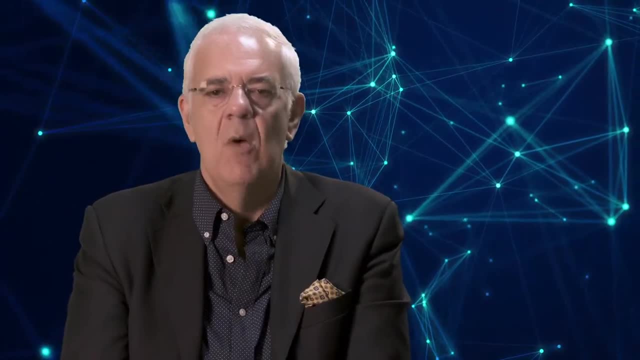 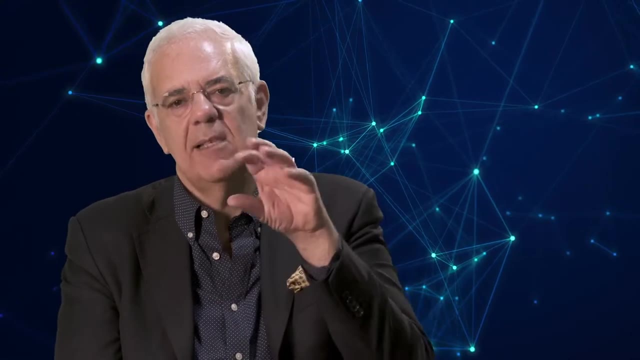 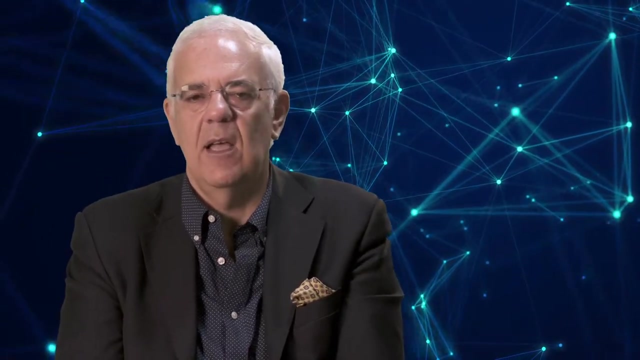 can have a square system of four n plus four equations in four n plus four unknowns. But the third solution is to solve. it can be shown to be of order n in which, on top of this, the system matrix has a three diagonal band. So you can use a simple Gaussian elimination technique to solve and find. 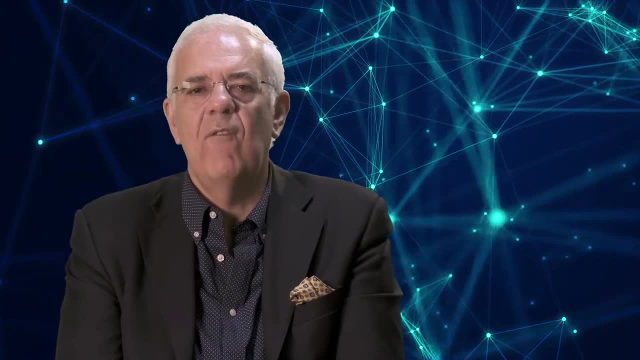 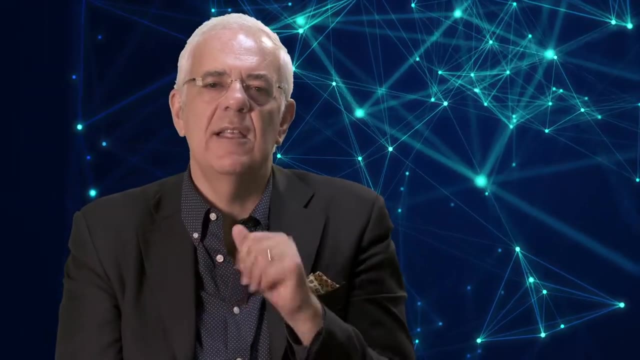 the solution. The fourth technique consists in, instead of requiring the passage through the path points, we can, we can have a passage through the via points, and and this via points can be achieved in two ways. One way is to have a technique of a linear interpolation with 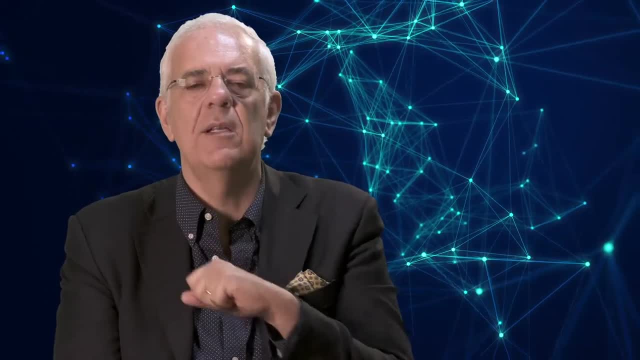 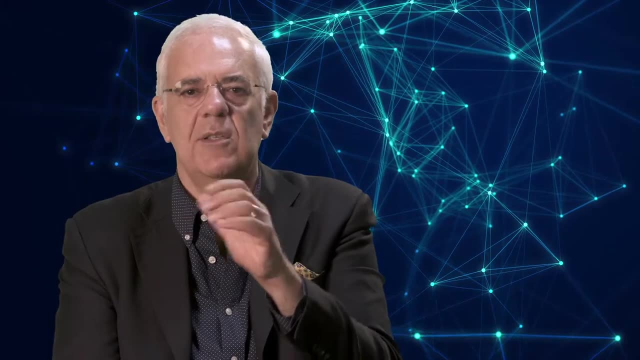 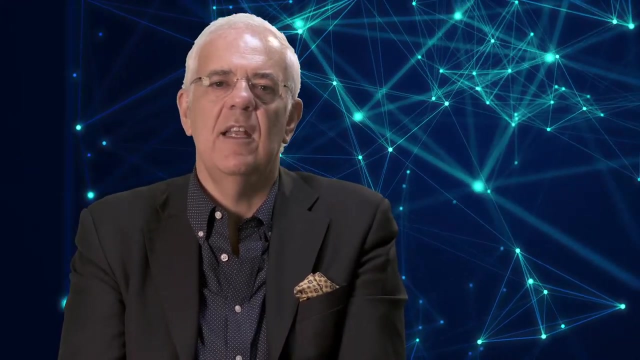 which the acceleration in around the via point is computed as the average of the two of, as as the sum of the square, the the average sum of the two velocities before and after the point. or there is an even simpler solutions, just resorting to the technique in industrial setting which consists 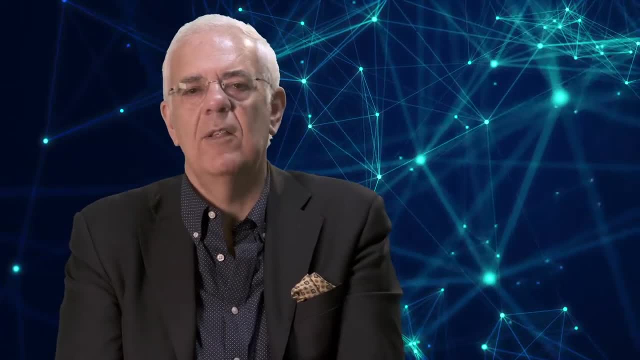 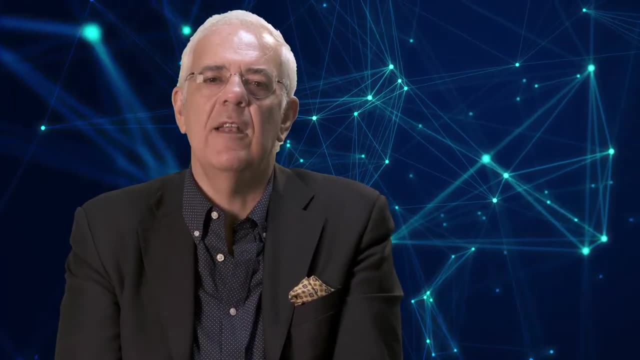 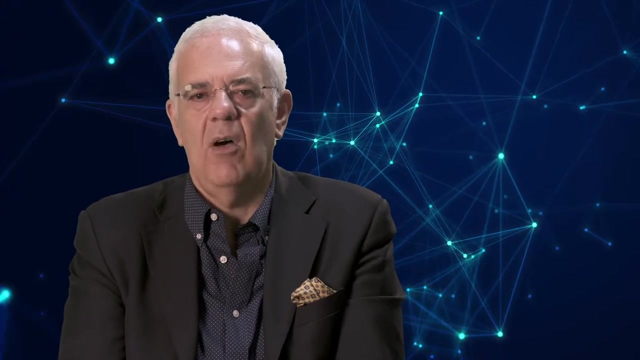 in anticipating the generation of the second trapezoidal velocity profile in such ways to gain time and to guarantee the flying motion through the via points. The final topic that we'll be considering in trajectory planning in the joint space is concerned with the dynamics of the robot manipulator. You remember the dynamic model for the first part.